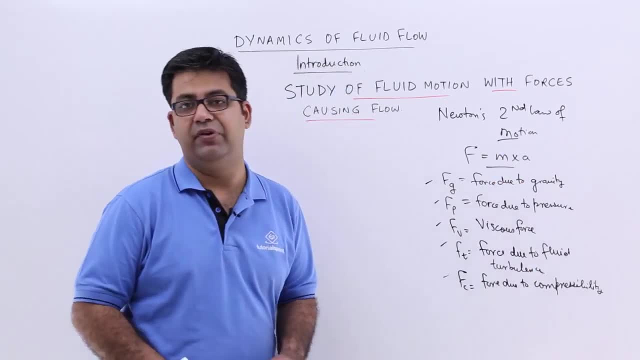 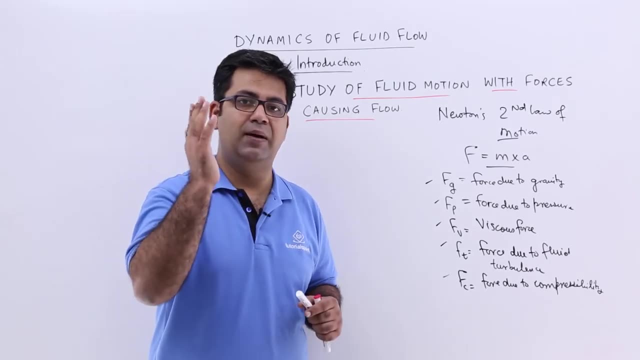 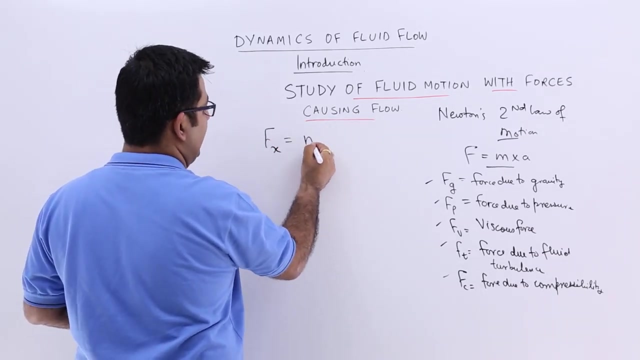 you can have 1,, 2,, 3,, 4,, 5, 5 different forces during a fluid flow. Now let us say that we are having a fluid motion in a particular direction, That is, let us say, x axis direction. So you will have the force in the x axis as m into. 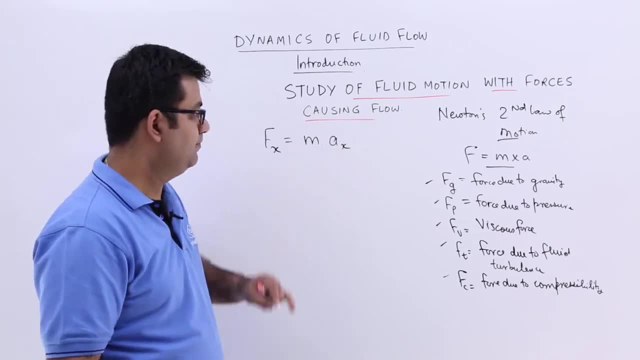 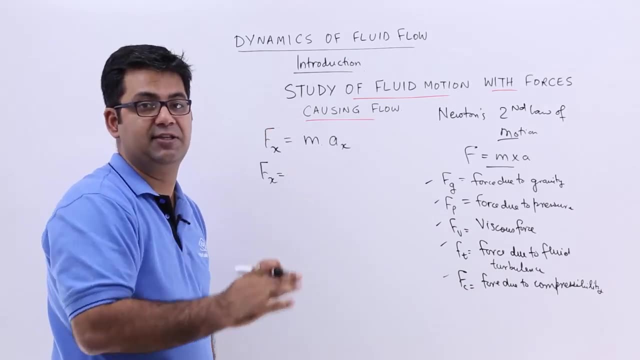 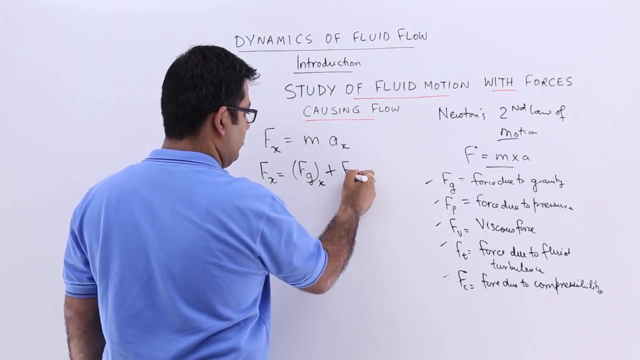 the acceleration component in the x direction. So if I have to write down that the total force in the x direction would be a sum of all these forces, yes, in the x direction only. So you will have the gravity force component in the direction x, the pressure force component. 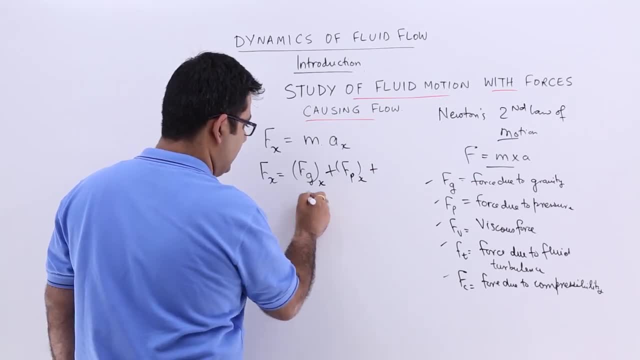 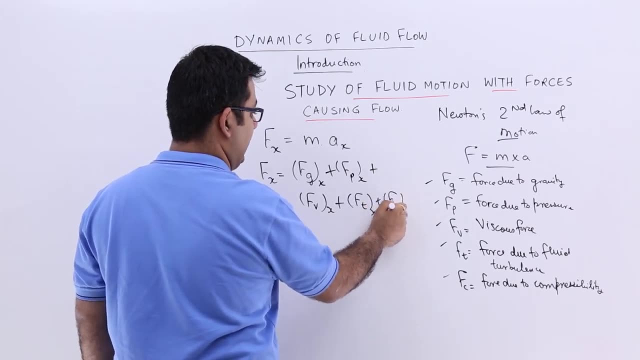 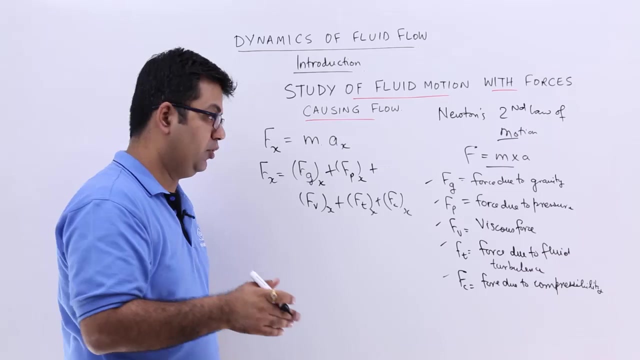 in direction x, the viscous force component in the direction x, the force component in the direction x. then you have ft of x and then fcx. okay, So this is the total force that can act during a fluid flow in the direction x. okay, So let us say this is the total force. 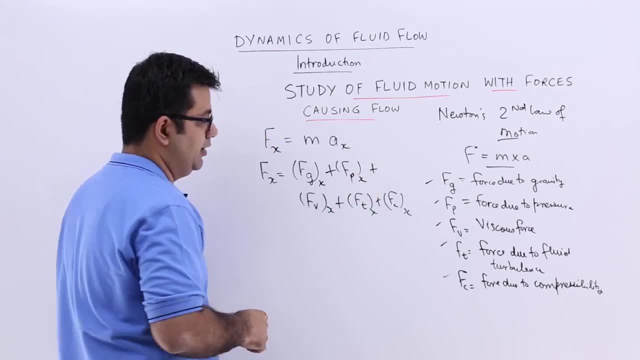 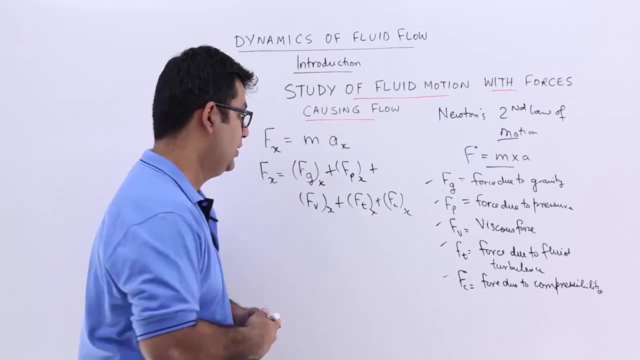 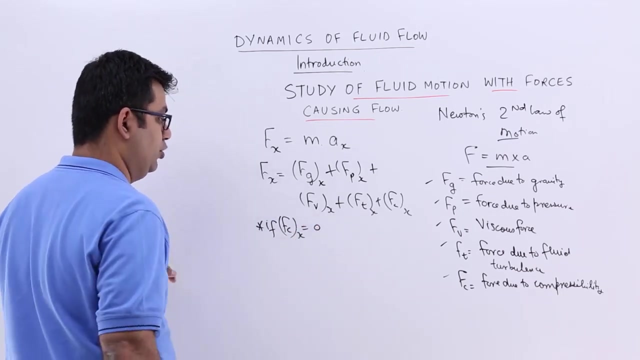 equation: If I assume that my force, due to compressibility, is 0,, that is, my fluid is incompressible, okay, So if fc in the direction of x is 0, or I would say, negligible, all right, this means incompressible. 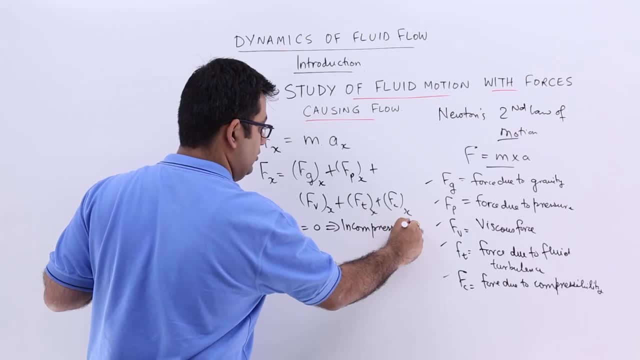 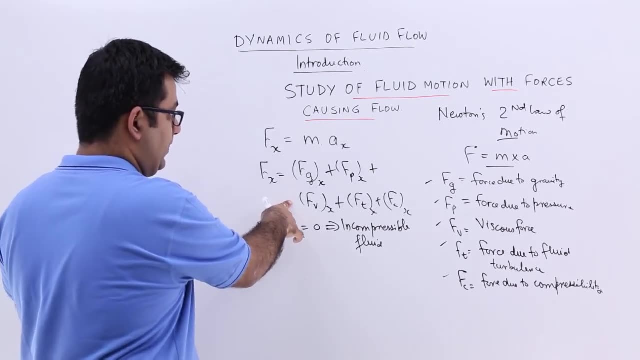 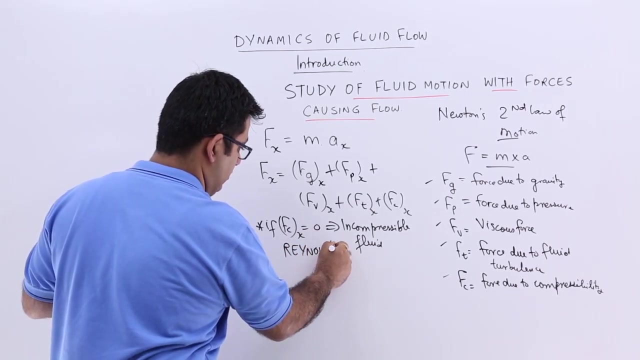 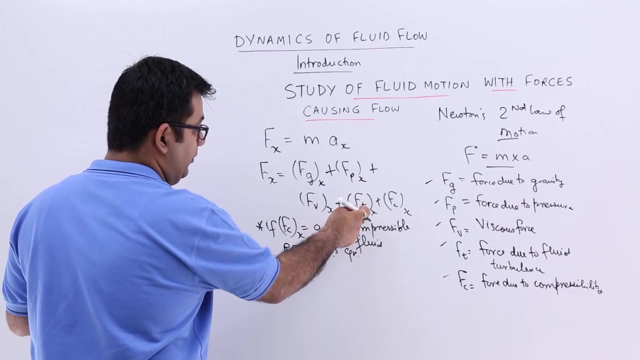 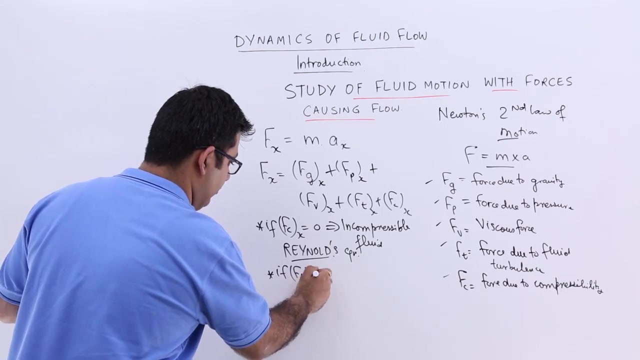 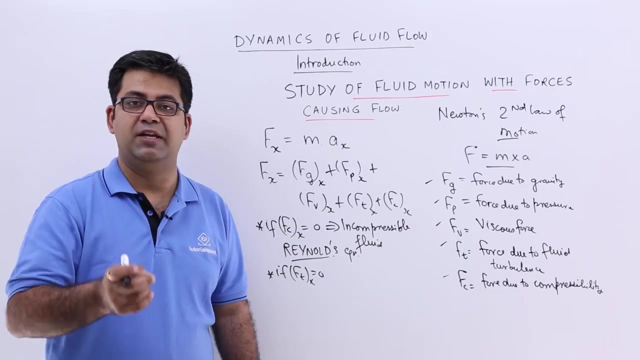 flow or incompressible fluid, all right. So when you put fc0 in this, the equation is called Reynolds equation, okay, Reynolds equation of fluid motion. okay. Now if I put the turbulence force also equal to 0, so if the turbulence force also becomes negligibly small, this means that the flow. 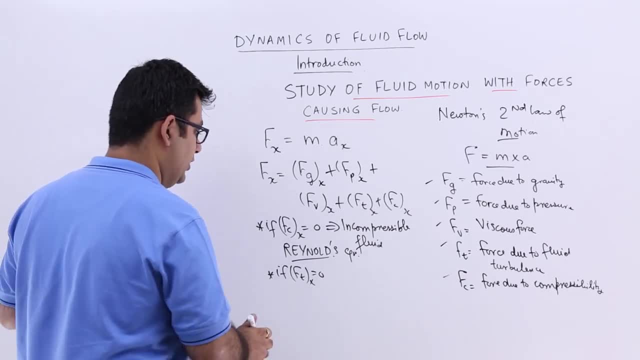 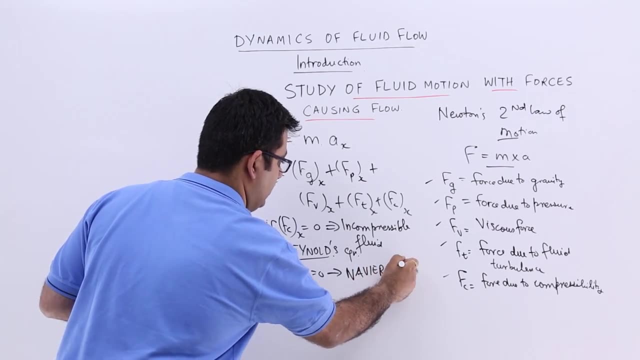 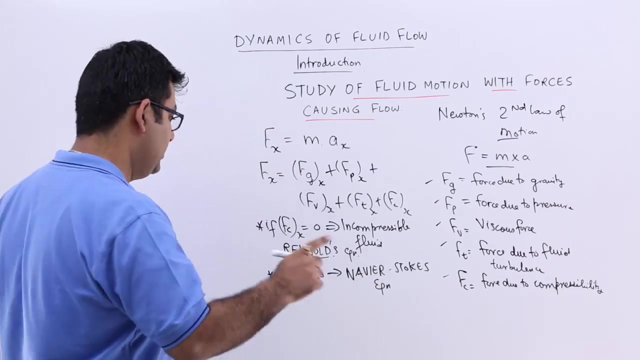 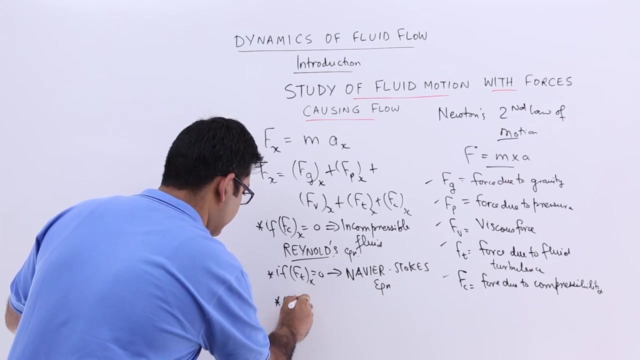 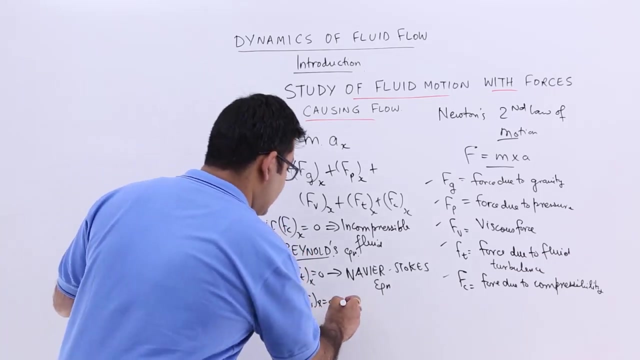 is not turbulent, it is laminar. then the equation is called Navier-Stokes equation, okay. Last, if I put the viscous force also equal to 0, okay. So let us say, if the viscous force in the direction x also becomes 0 or negligible, then the resulting equation is: